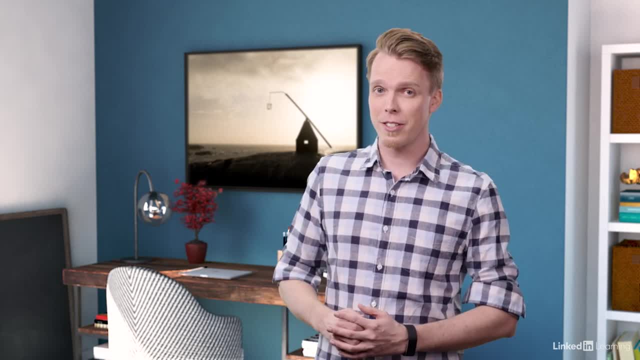 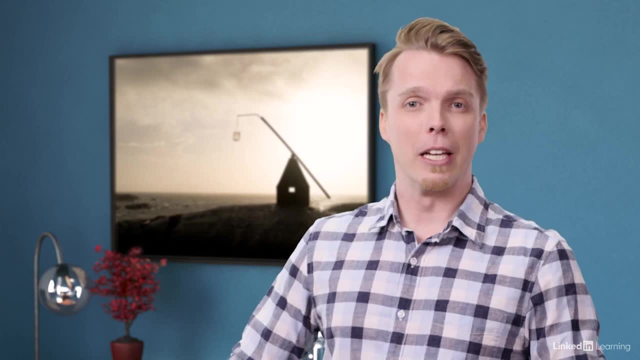 enough if we're doing something really basic, like simple math equations, but gets much harder when we're running more complex operations. JavaScript scripts can easily end up being hundreds, if not thousands, of lines of code, and we need some way of making sense of it all. 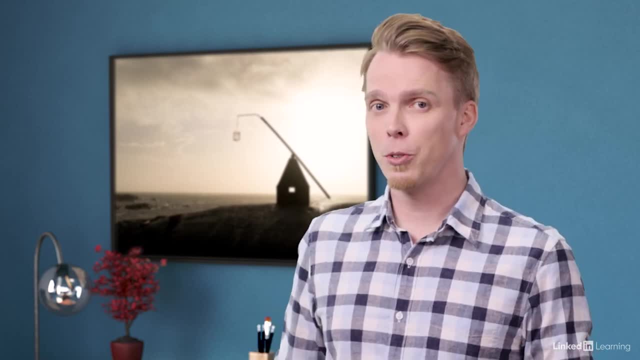 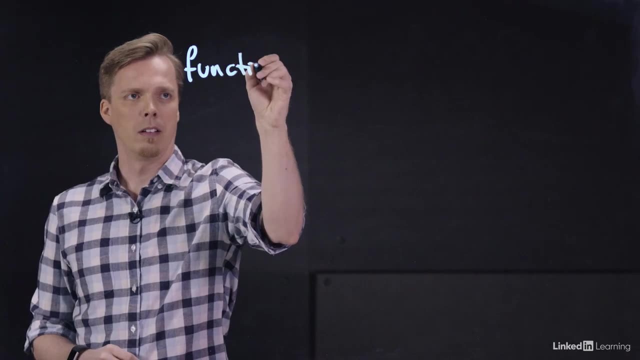 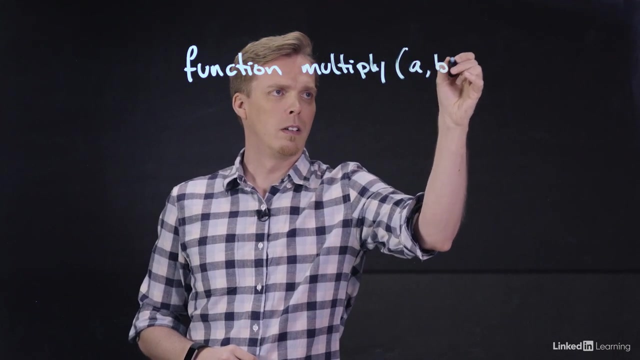 To help structure our code and make common operations reusable, we create functions and objects. Functions are mini-programs inside our scripts. They can be used to segment off sections of our code to make it easier to manage or to run repeated operations or both Functions wrap. 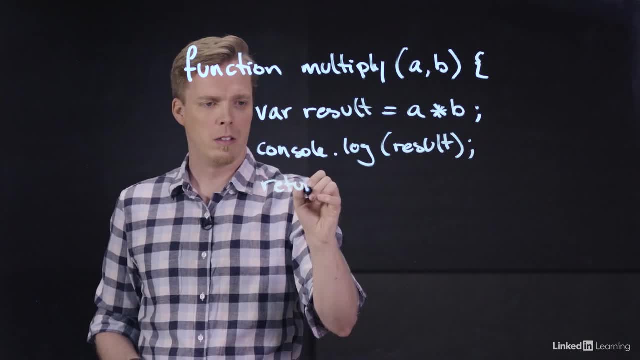 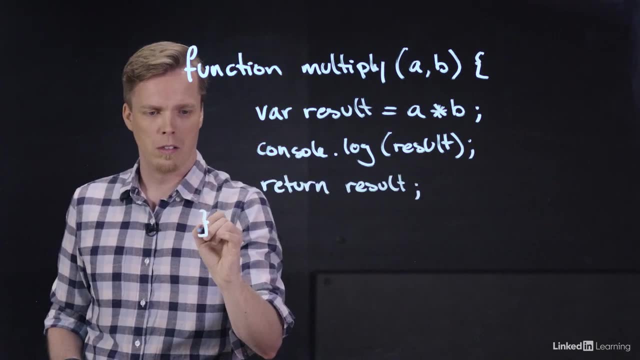 around code blocks which contain the actual statements to be run and typically include some common sense of how to do it. If we want to make it easier to manage, we can use a combination of variable assignments, operations and conditions. Functions do one of two things. 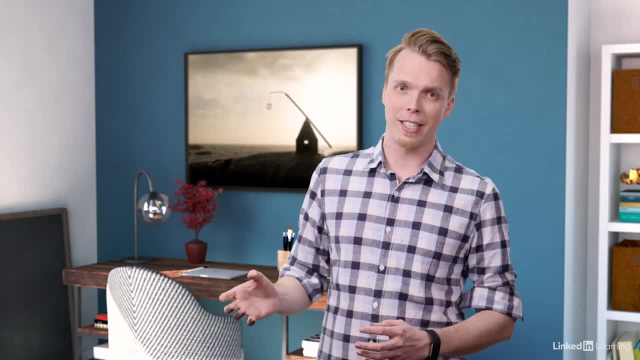 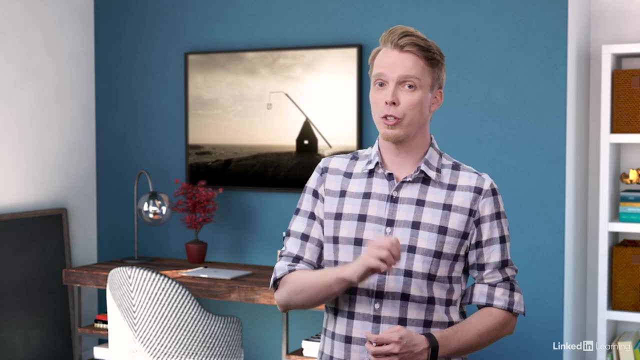 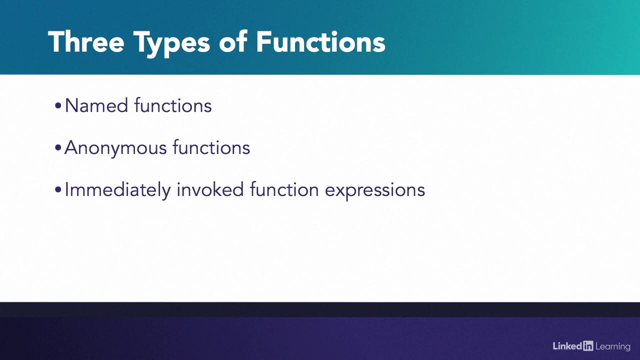 Either create a result immediately, like change the contents of an element on a web page, or provide an answer or output to be used by other functions called a return value. In JavaScript, we work with three types of functions: Named functions which are executed. 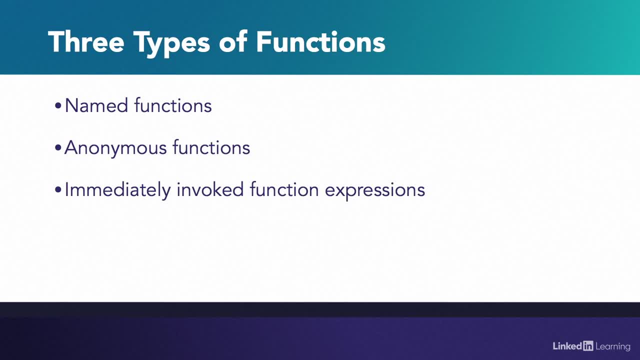 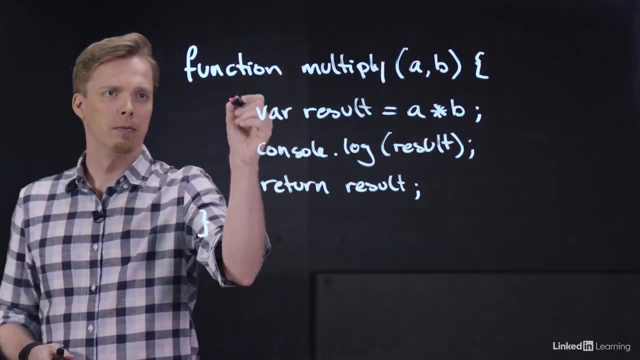 when called by name. Anonymous functions, which typically run once they are triggered, And we work with three types of functions: Named functions, which are executed by a specific event, And immediately invoked function expressions, which run the moment the browser encounters them. All functions have the same overall structure. They start with the 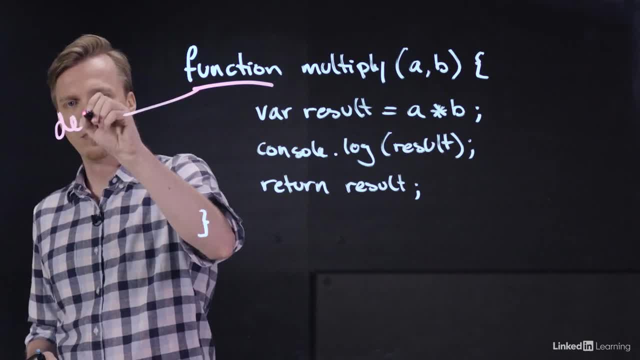 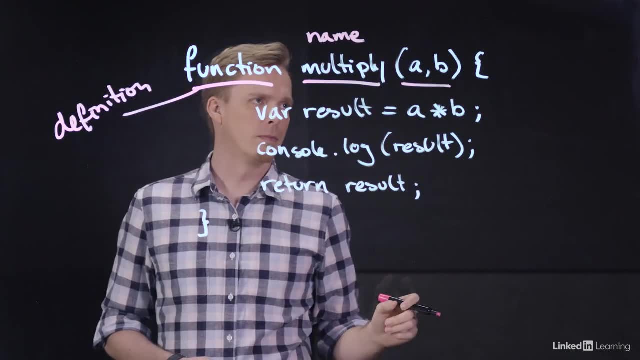 word function which tells the browser- here I am declaring a function, followed by their name, two parentheses and then a pair of curly brackets which wrap around the code block To run a named function. we call it by its name. 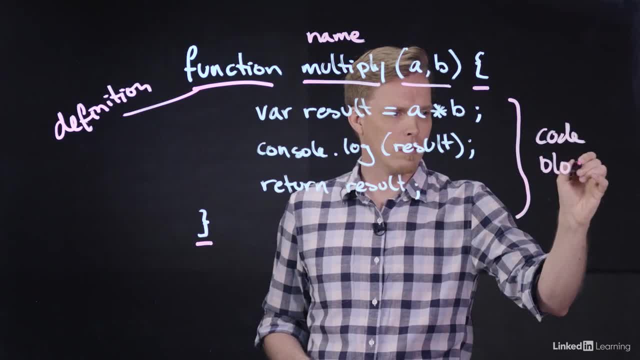 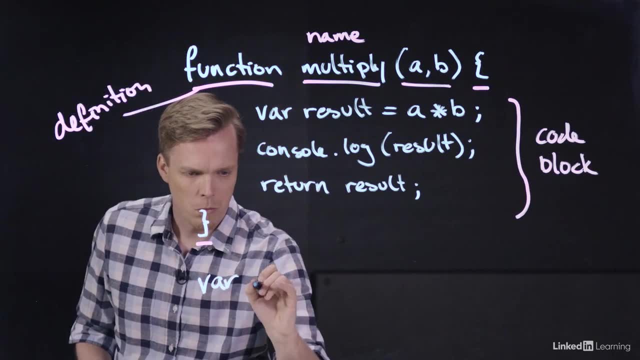 at the location in the script where we want it to run. That means we can define a function at the very top of the script and choose to run it at the very bottom of the script. In fact, this is the coding standard for functions. Technically, it doesn't matter where in the 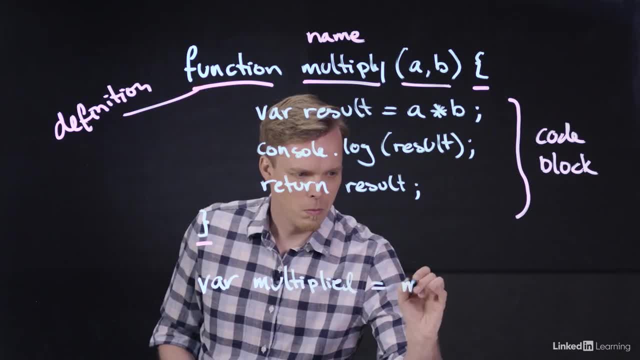 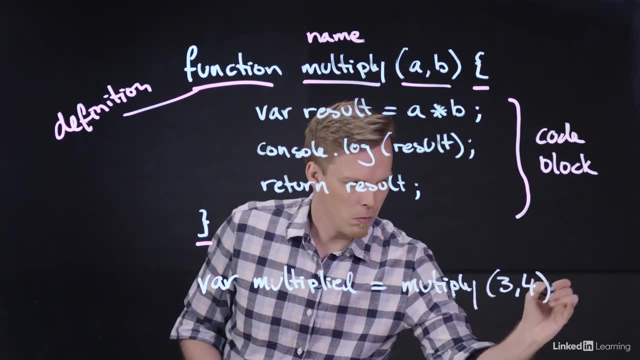 script a function sits because the browser will load all the JavaScript first and then run it. But for readability for humans, we typically place a function before it's called in the script. This provides a semblance of logical structure in our code when you're reading.